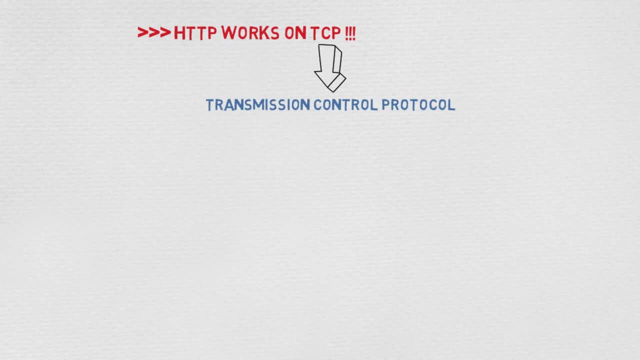 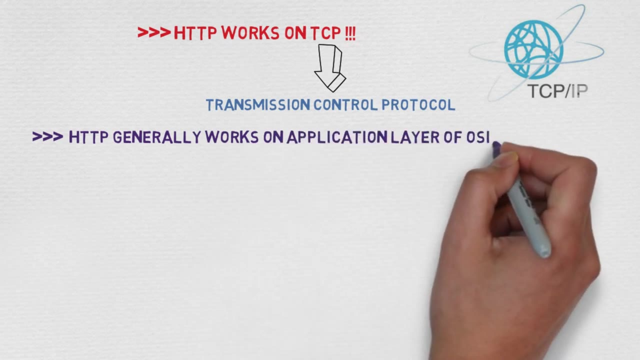 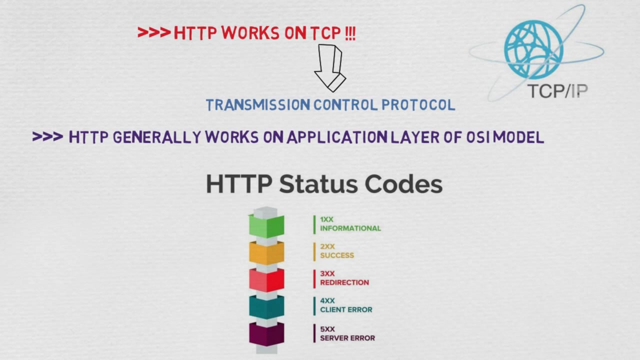 HTTP works on TCP. TCP is Transmission Control Protocol. TCP is Stateful. HTTP generally works on the application layer of the OSI model. Now HTTP status codes: Any codes with the string 1 are informational Codes. with a string with 2, convey successful response. Codes with 3 indicate redirection. with 4, client error. and. 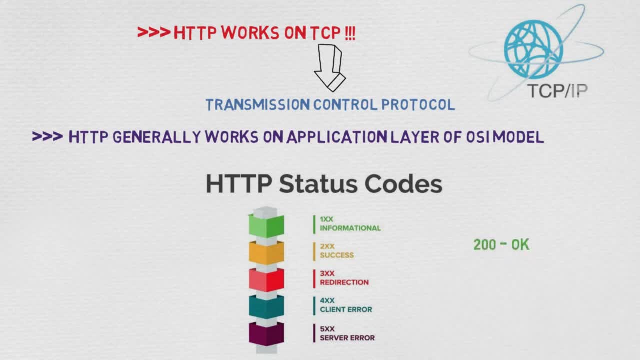 with 5 server error. So, for example, code 200 indicates OK, that is successful response And page 404 indicates page wasn't found in the server's database. So, for example, code 200 indicates OK, that is successful response And page 404 indicates: 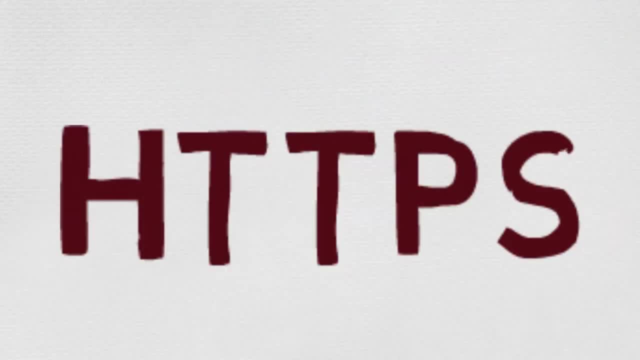 page wasn't found in the server's database. So, for example, code 200 indicates OK, that is successful response And page 404 indicates page wasn't found in the server's database. We have known HTTP. now What's HTTPS? HTTPS refers to Hypertext Transfer Protocol. 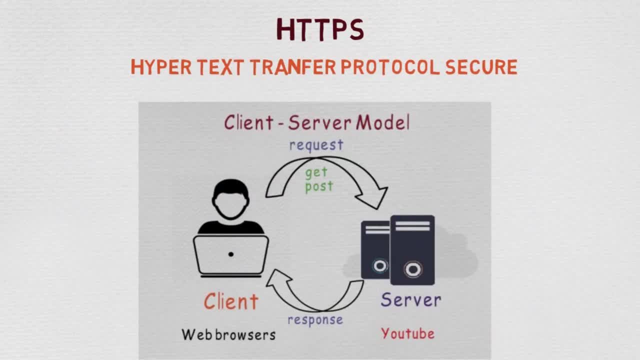 S for Secure. So the same client-server model exists here, but a small difference is both client and server have keys And when the client sends a request, he or she logs up his request. So a server with the key can only access this request and response is also. 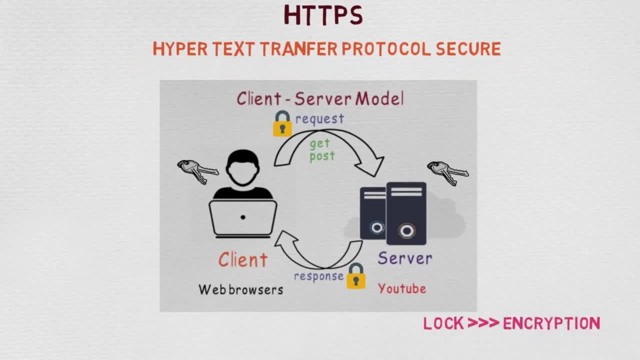 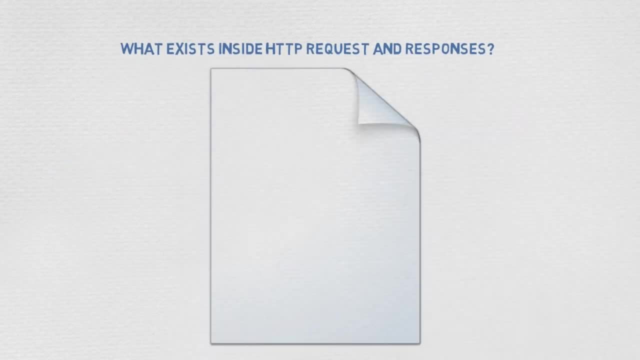 logged up. Log refers to encryption. Now, what exists inside of the HTTP request and response? Both are just some text files. In this file, this small portion is HTTP header, followed by a blank line which is just for separation between the contents. Then comes 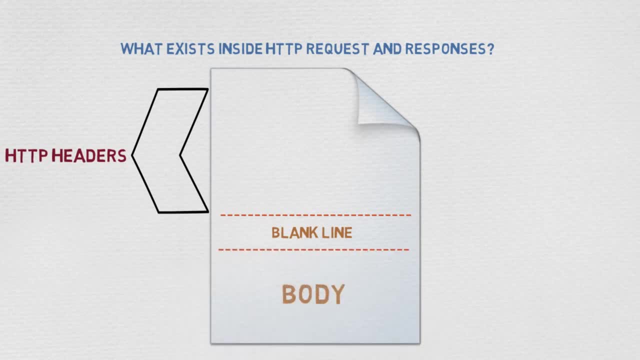 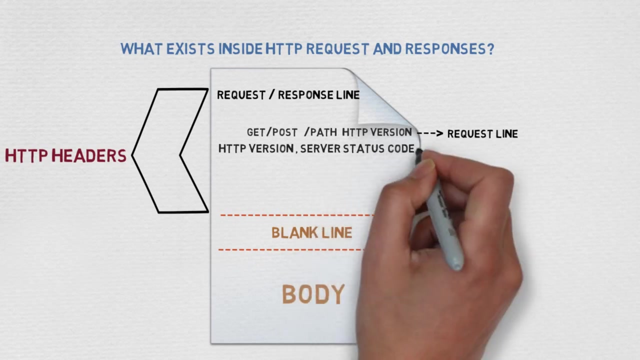 the body. Body is just additional information Coming to HTTP headers. now. First is the request or response line. In request line, GET or POST method and a path of the requested file including the HTTP version is used, And response line consists of HTTP version and server status. 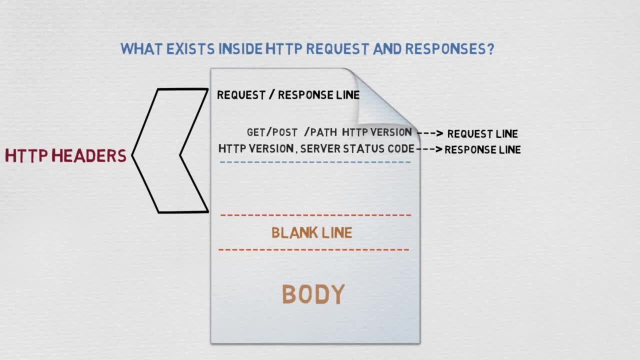 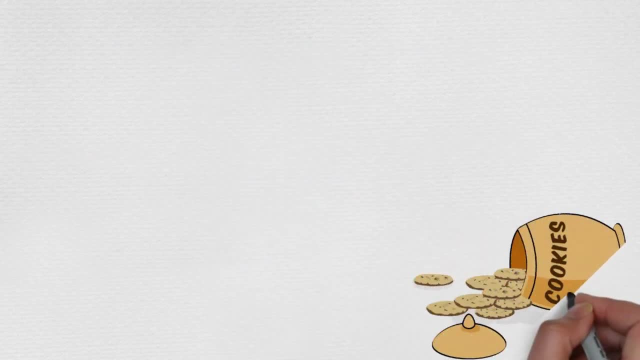 code. So the HTTP header is the HTTP header and the response line is the HTTP header. So the second one is optional request or response headers, which are basically name value pairs. Moving on to cookies: Wow, yes, these are yummy, But, guys, I'm sorry these cookies. 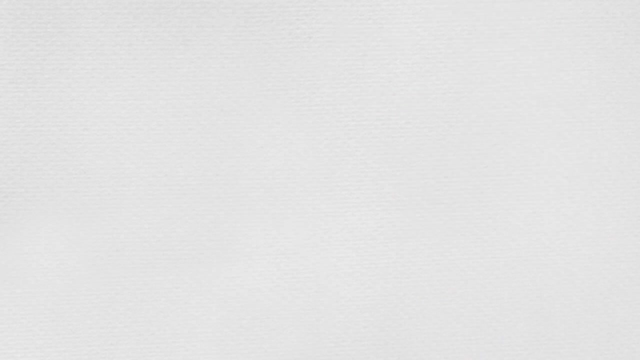 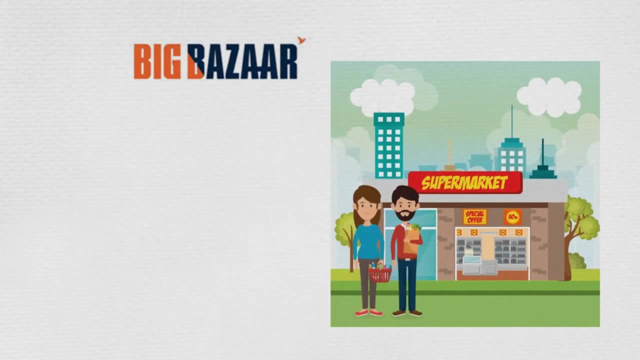 are not what you're thinking. I'll tell you what are these. now. Let's suppose you visit a supermarket near your home regularly. That supermarket is a big bazaar. You go there, you buy things regularly, but that store doesn't remember your details, exactly like they don't. 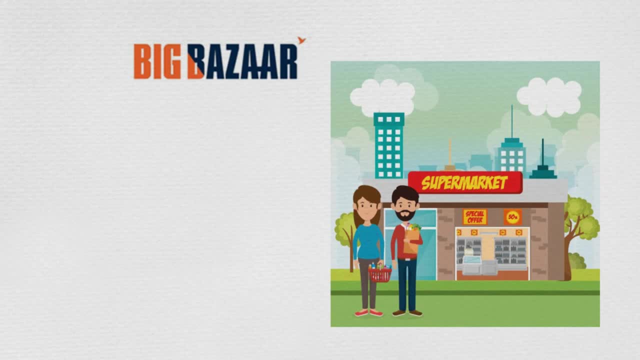 remember the things you have bought previously, etc. etc. This is a stateless relation between you and the big bazaar. But you have a problem now. You wish to exchange some things you have purchased previously. Now the store can't trust you. It doesn't exactly know. 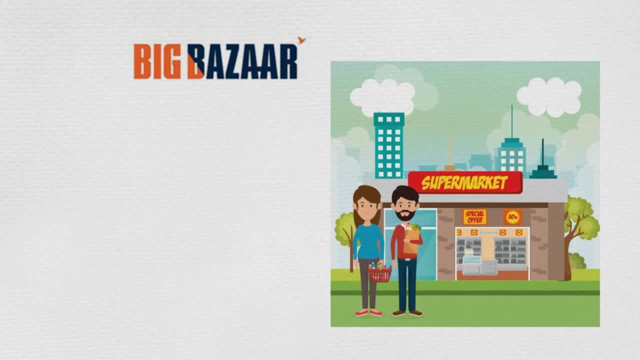 if you have bought that particular thing from them or not. So for this exchange process you need to have a stateful connection with the big bazaar. So to solve this problem, the store has given you a membership card And if you scan it with them they can insert. 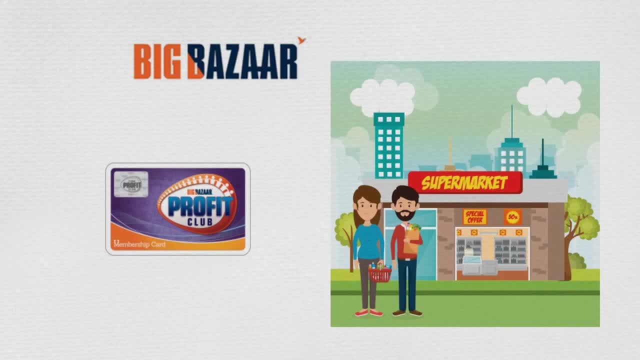 your details instantly, trust you and exchange an item for you. So this membership card here provides a stateful interaction. Now let me tell you the analogy of this concept to the internet. Big bazaar is a server, card is a cookie and you are the client. An important 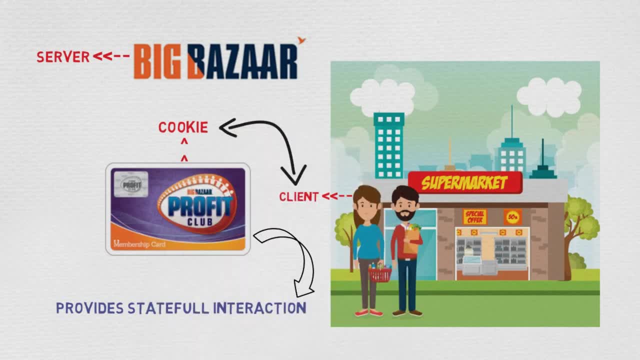 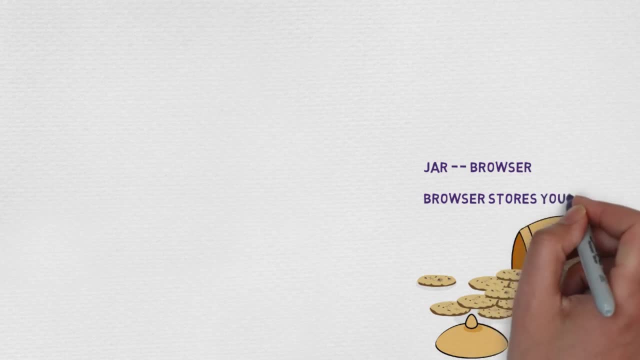 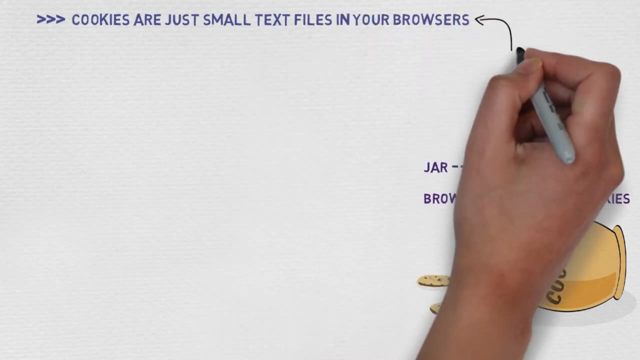 thing here is: client has or stores the cookie. That is, you have the card with you, But in technical terms browser is the client, So browser stores cookies. Cookies are just small text files in your browsers. They are stored in the browser's. 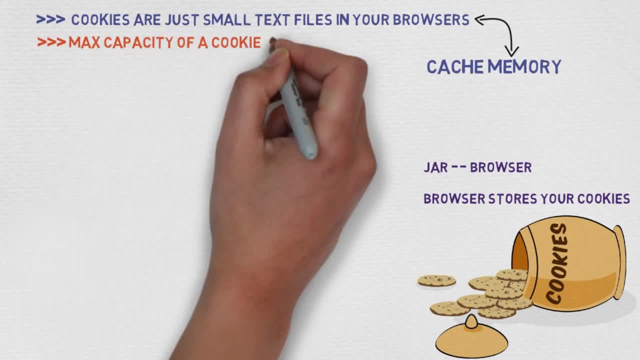 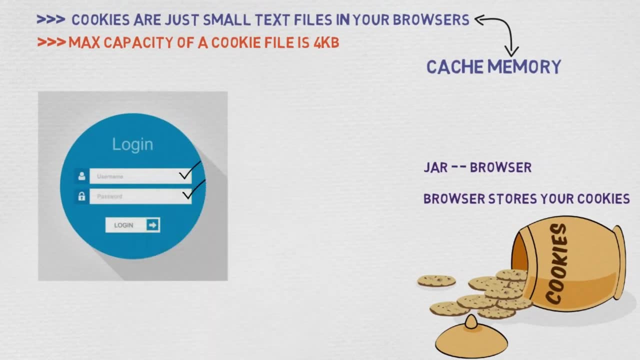 cache memory. Maximum capacity of a cookie file is 4 KB. So let's understand how cookies work. First, suppose you have a login screen where you have to enter your username and password. This action means you have submitted your details to the server and requested for. 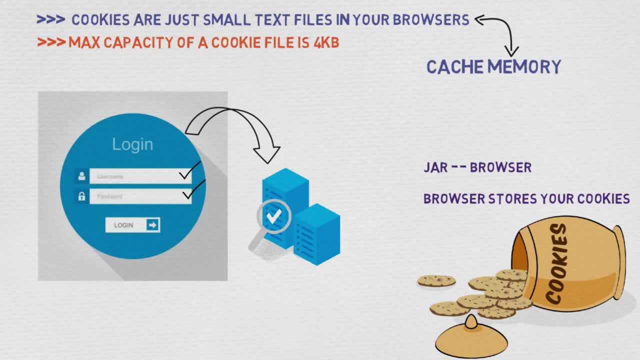 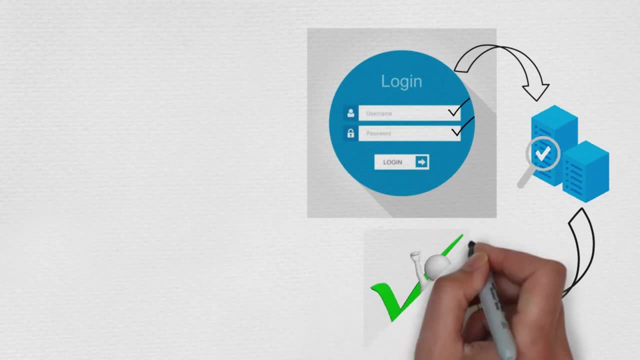 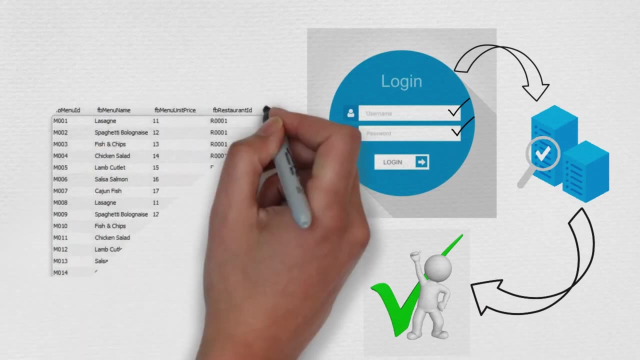 your login into the website. Then the server validates your details against your database. That is, it needs to check whether you are the correct user whom you are pretending to be or not. For validation, the server goes to its database, searches for the details you have submitted. 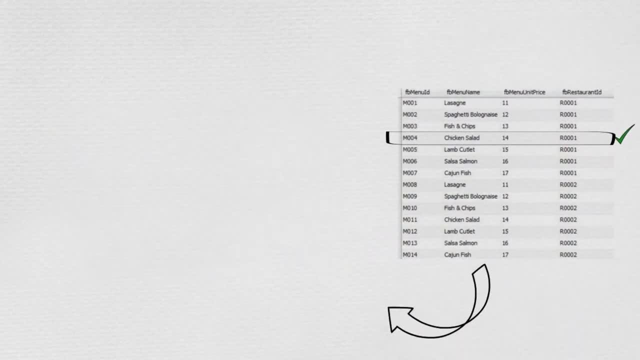 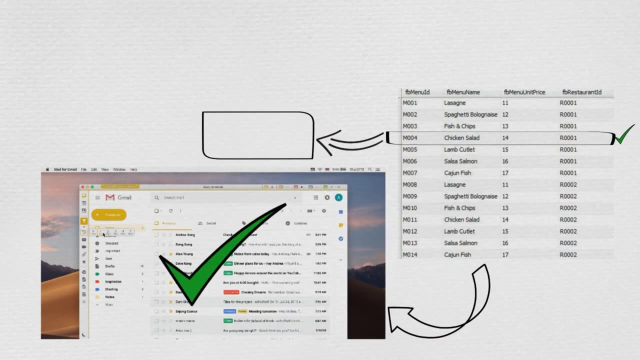 and validates it. Then, if they are correct, the server responds back to the client with a log-in screen. Now the server generates a session id against your details in its database. This session id is stored inside a cookie in your browser. The session id is randomly. 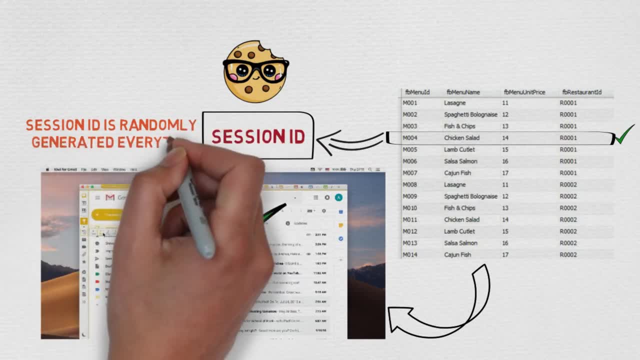 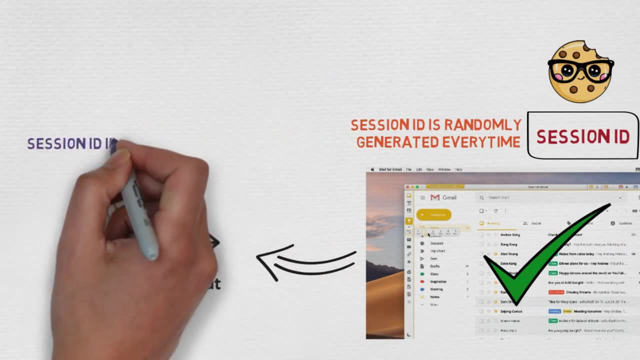 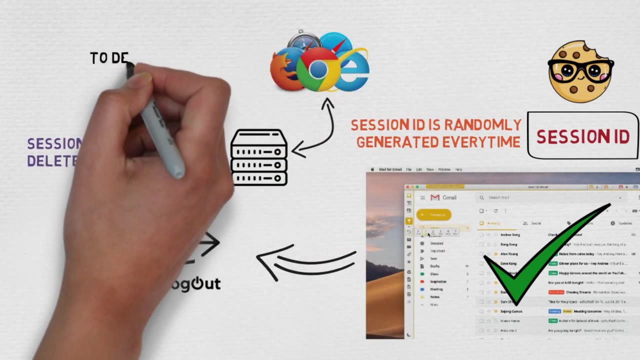 every time you log in. then suppose, if you log off from that website, the randomly generated session ID is deleted from the server. as you have logged out, the server also instructs your browser to delete the details of that particular session ID. so finally, unless you log out, you need not use username and password. 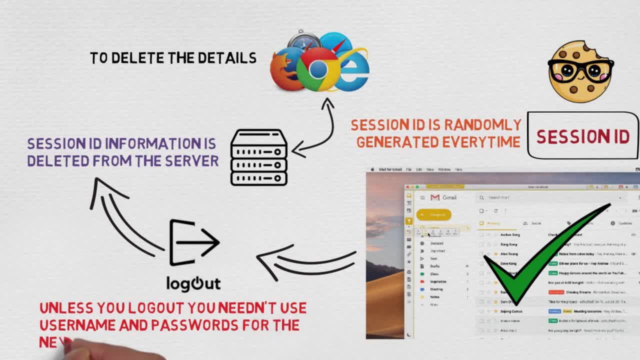 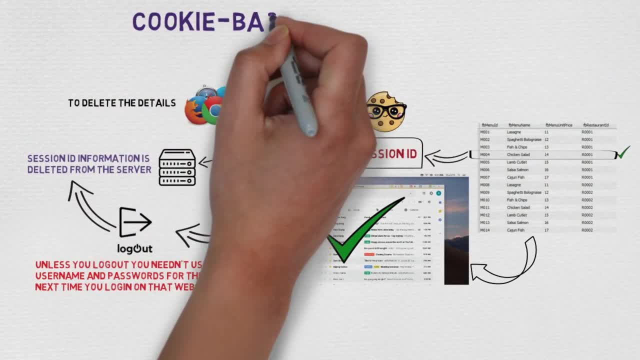 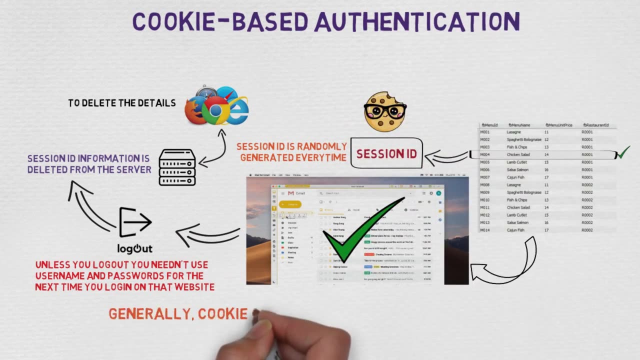 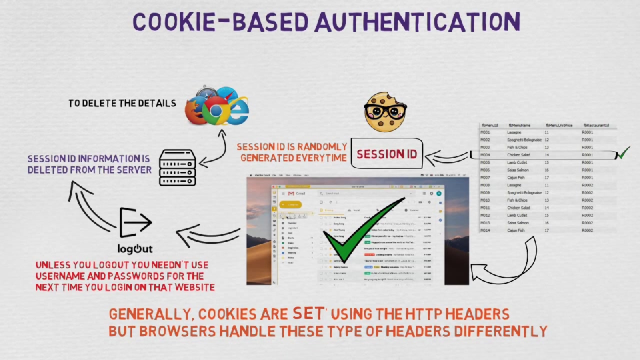 for the next time you log in on that particular website, so this is called cookie based authentication process. generally, cookies are set using the HTTP headers, but browsers handle these type of headers differently, so let me now show you all these HTTP headers, cookies, sessions, IDs and different ways you can. 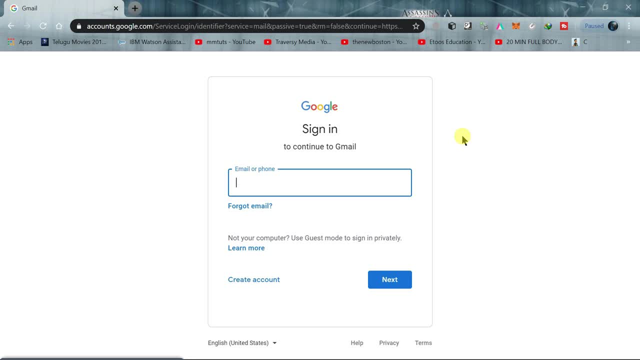 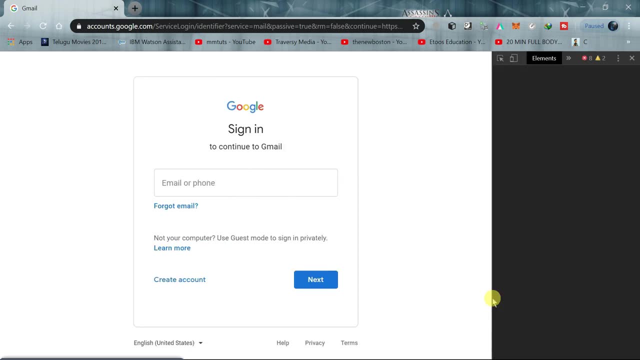 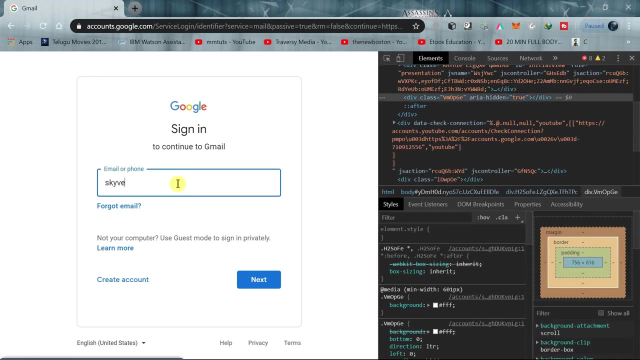 view the cookies accessing your browser at the moment, practically just right click on the browser and click inspect. then let's login into the main. that is Gmail login screen appears here. this login into that giving your username and password. now we do not need an inbox screen, so let me make the inspect element bigger. 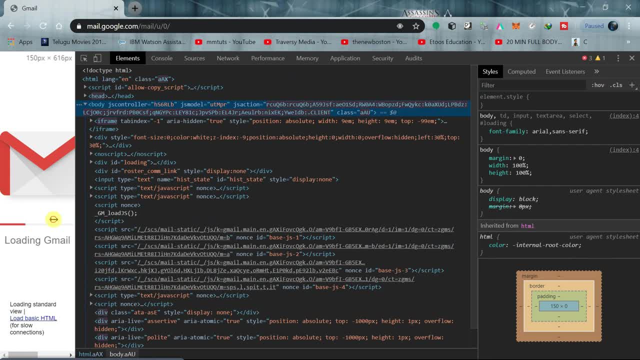 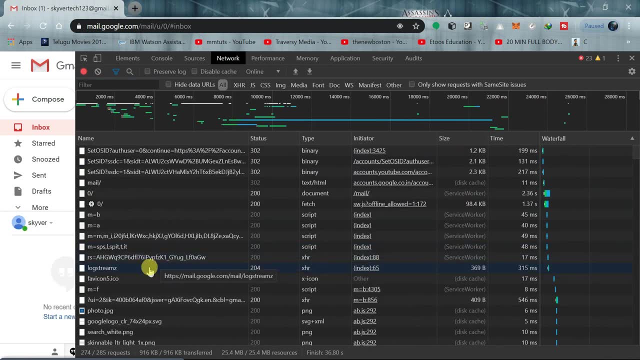 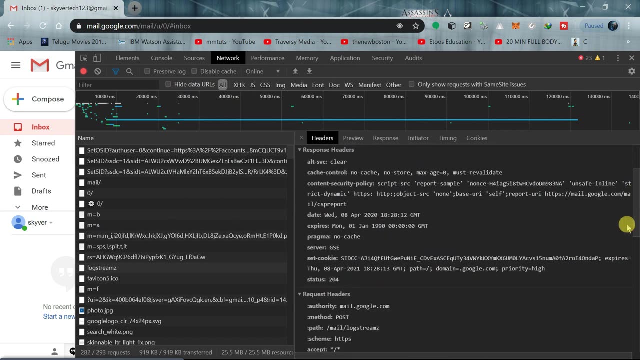 and then go to the network tab here. here you can see all the network traffic. there is all the files as the server is sending and responding back to the client. so now let's find the login access granted file here. if we observe here in the header section, then jot Z 선생님, above nothing, then the in the 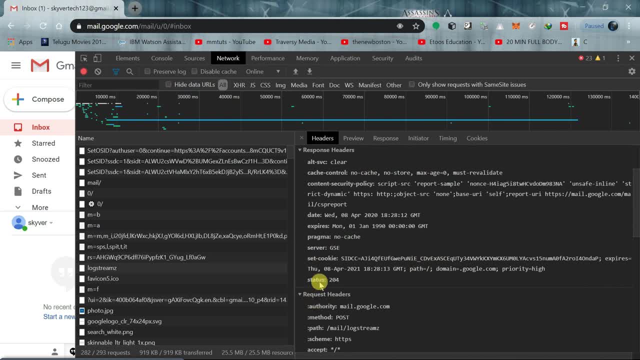 headers section there is response headers. right now I forgot the server person. there you can find the server. if the screen wolver line exists, mainly be the dot fors and in other certain cases the attacks selected at the, which is a success code and the cookie is actually set by the server using the. 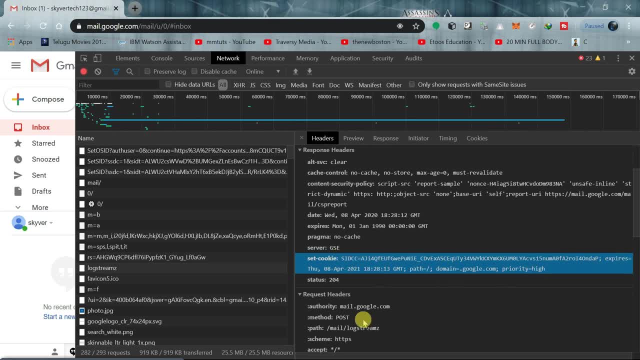 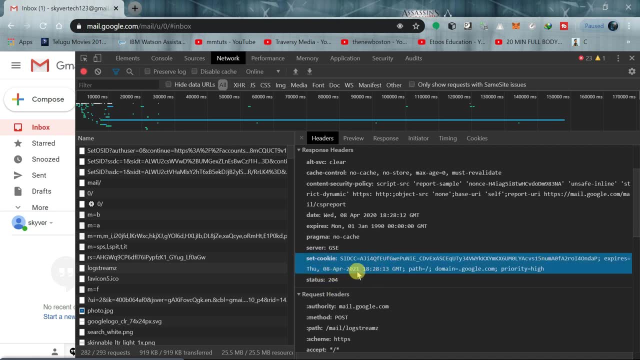 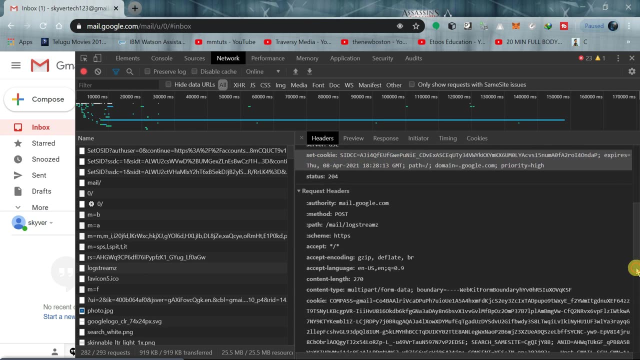 set cookie attribute. inside cookie we have session ID, the expired date set and the domain. if you log out from the Gmail before this expired date, the cookie will be deleted automatically from the server and the browser respectively. then we have the request header in which there's post method, in this case the path and. 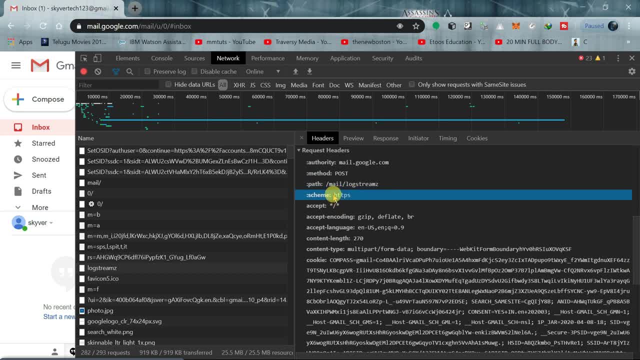 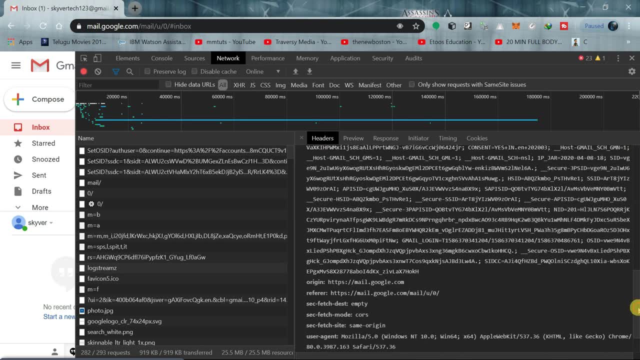 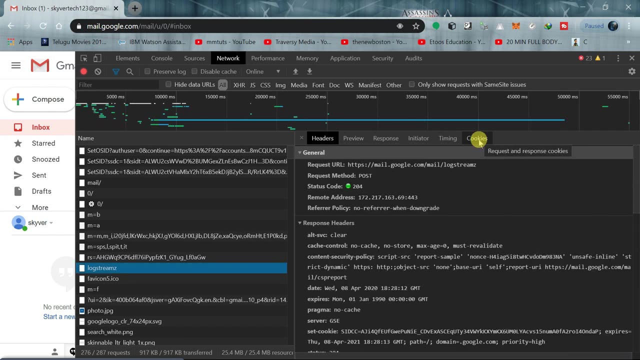 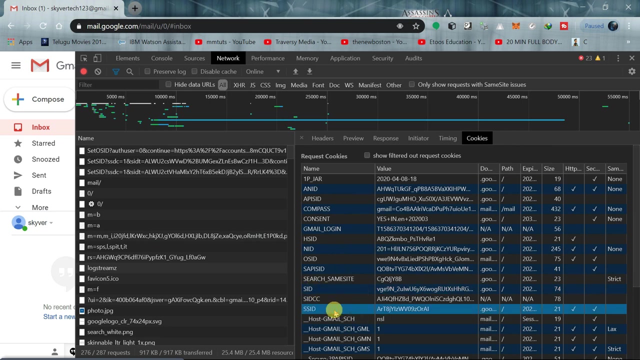 the HTTP version. others address the in value pairs, that is, optional headers. now go ahead and click the cookies section here, or you can see the SID and SSID, where SID refers to the session ID, but here there are two as ideas, that is SID and SSID. what do they refer to? Sfon ID is aард oppressor to sid on your website. tooth suspension related to how you can edit Valley and location Id. the pre petition is shipping to the seizo site of the machine user to copy mail order in the piso or email to theими terminal zao ad. 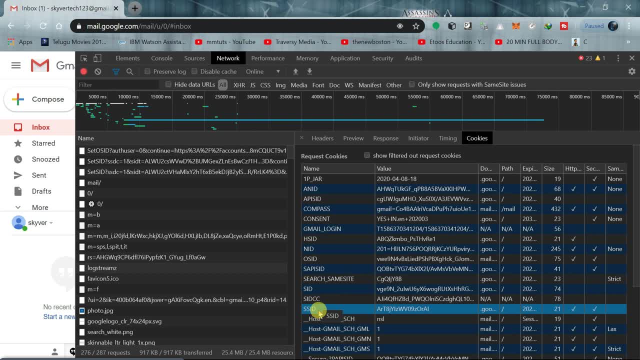 P bar. there is a search bar. you cannot install it if you wish to Getting the�� in. SID refers to the HTTP and SSID refers to HTTP version. so they are just different versions. If you observe here, both the session IDs are in encrypted formats so that they can't be. 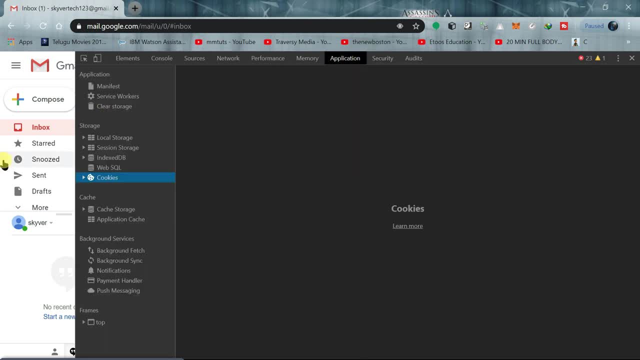 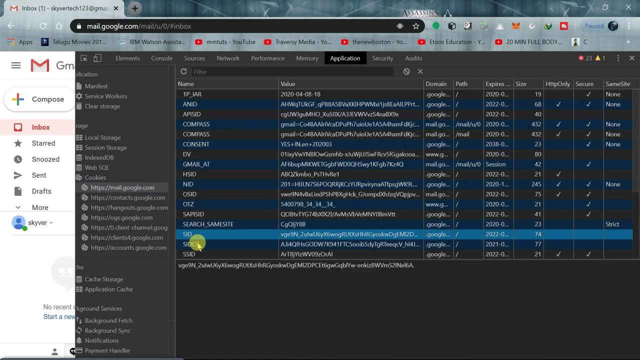 hacked easily. Second way you can view cookies in the browsers is through application tab. Under this, go to the cookies and select Gmail. So here also you can see the same SID and SSID, which are in the encrypted format. So go ahead and close it now. 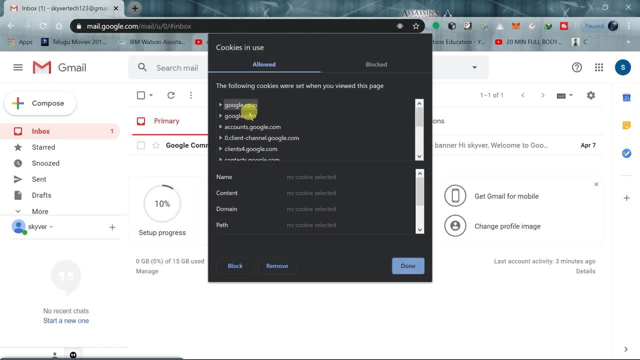 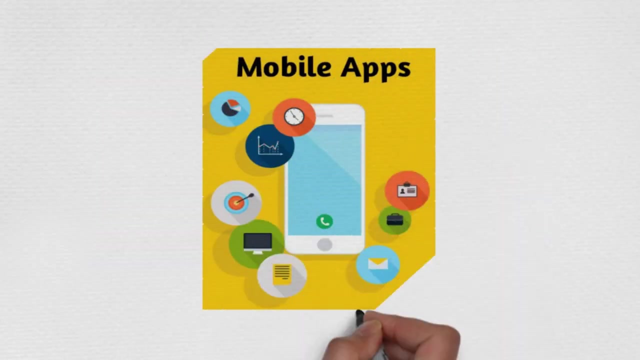 And the third method is click the small lock icon here in the address bar. Under this you can see cookies section, Then go to mail and then cookies again. here also you can find SID and SSID. So that's it for this practical Moving on to tokens. now let us consider you wish to use a mobile app, which you need to. 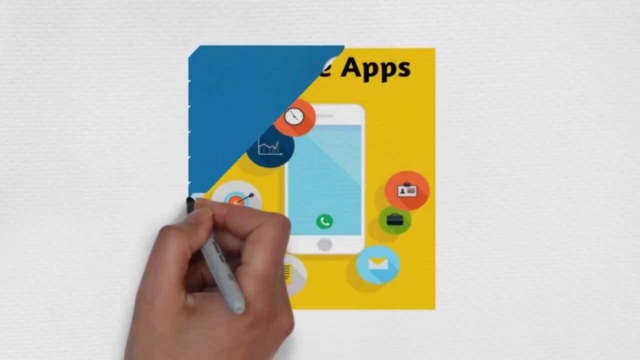 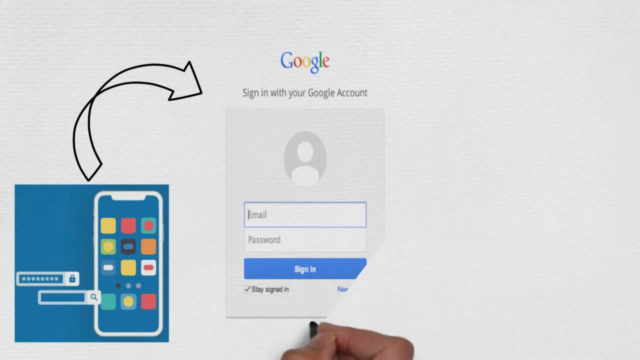 sign in, But you do not trust that app to give your username and password. So when you click to sign in here, this mobile app redirects you to a Google website where you can provide your details, as you trust Google. Then the Google asks you: hey man, do you like to give this app grant access? 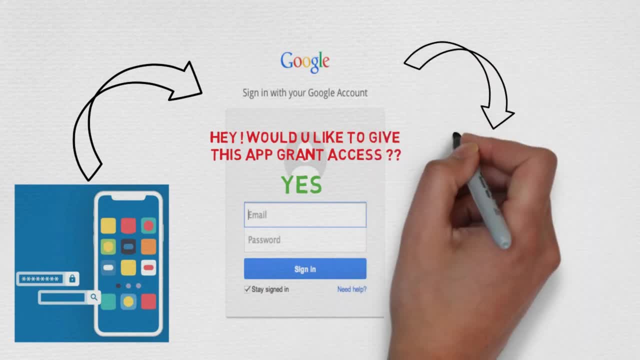 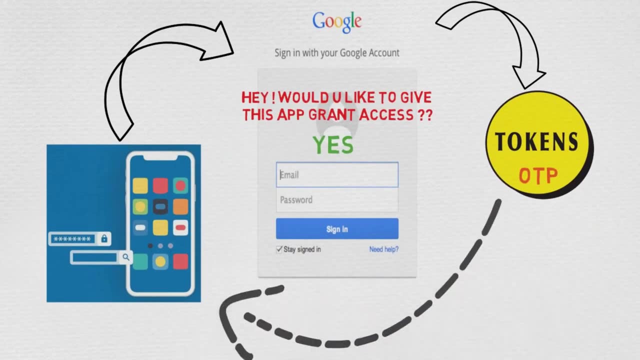 If you click yes, the Google server then generates a token. This token is just an OTP like one time using. This particular token is sent to the mobile app and now you can access your Google account in that particular mobile app. Here you need to notice that tokens do not contain your username and password. Here you need to notice that tokens do not contain your username and password. Here you need to notice that tokens do not contain your username and password And hence they can be trusted for authentication. Popular token based authentication processes are OAuth, OpenID and JWT.